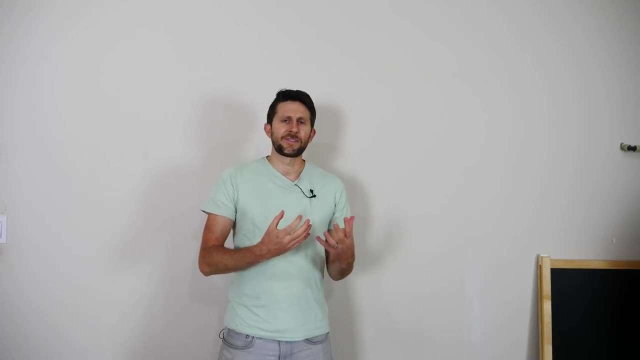 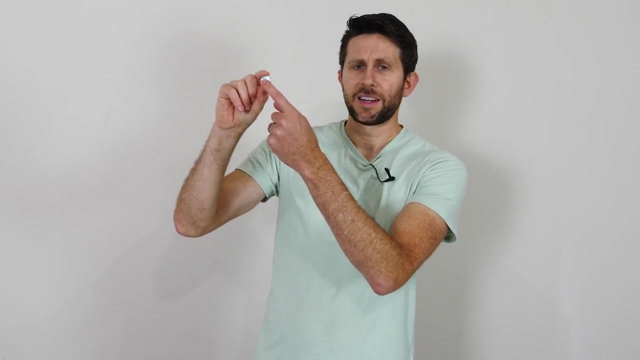 total is going to be 350 exactly. So where does the 35 number come from? with a six-sided die, Let's get a really easy dice like a coin. So if I have a coin here and I write one on one side and two on the other side, that's basically a two-sided die And I flip the coin. So let's say: 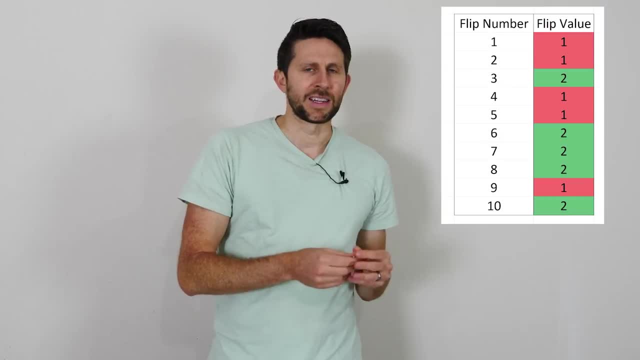 I flip the coin 10 times. About half the time I'm going to get one and about half the time I'm going to get two. So if I add up the total number that I get, I'm going to get all the ones plus all the. 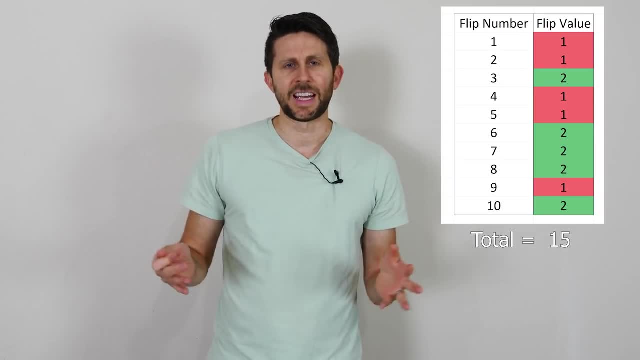 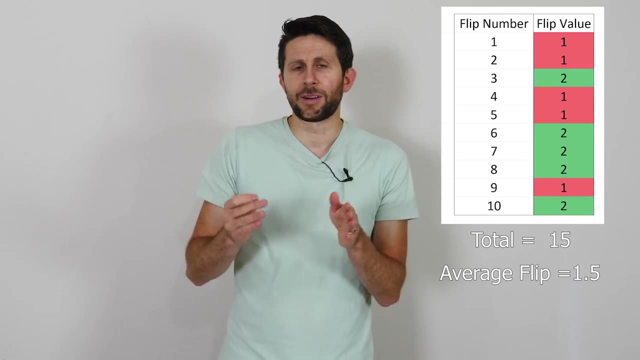 twos. So that's five ones and five twos And if I add those all together that's 15.. And I flip the coin 10 times. So on average I got 1.5 per flip. So the 1.5 comes from taking the average between: 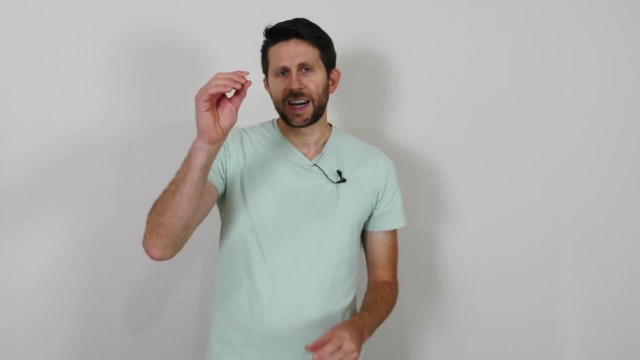 one and two, which is 1.5, halfway in between. So I'm going to flip the coin 10 times and I'm going to take the average between. But a dice doesn't just have two sides, it has six sides. So you take the. 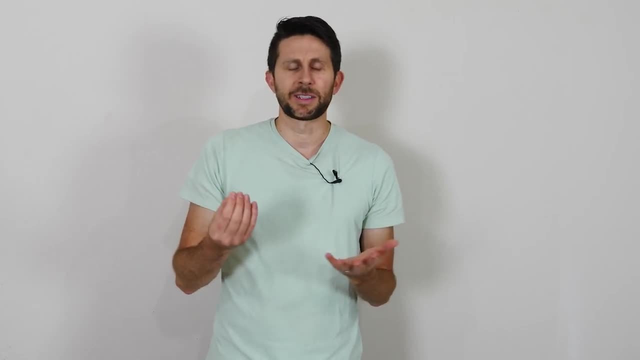 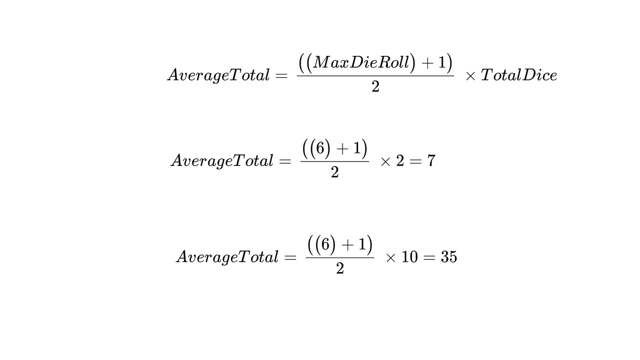 average between one and six, which is 3.5.. And then you just multiply it by however many dice you have. So that means the most probable number to get with two dice is seven. The most probable number to get with 10 dice is 35.. So that's how I came up with 35, when I guessed the most probable. 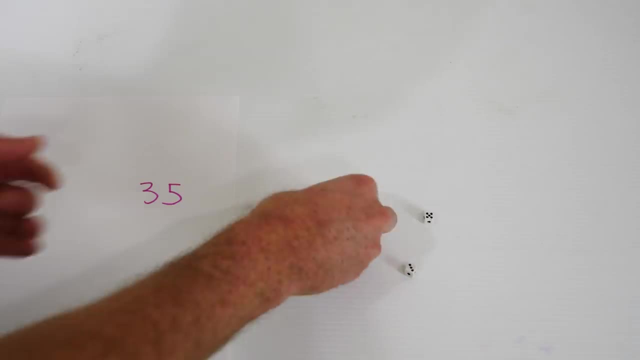 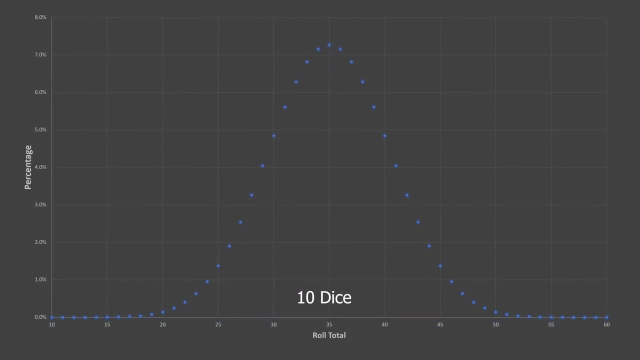 number that the total number of dice would equal. So I only had to do a few rolls before, sure enough, I got 35. But if you're ever trying to guess the total roll of a certain number of die, remember that the more dice you have, the more tight the probability spread is The less dice you have. the more wide it's spread. So why does that middle number end up being the number that's chosen the most? It's because of all the permutations of numbers you can get on. each of the individual die. there are more ways to add up to a number that's right in the middle, For example, to roll a seven. 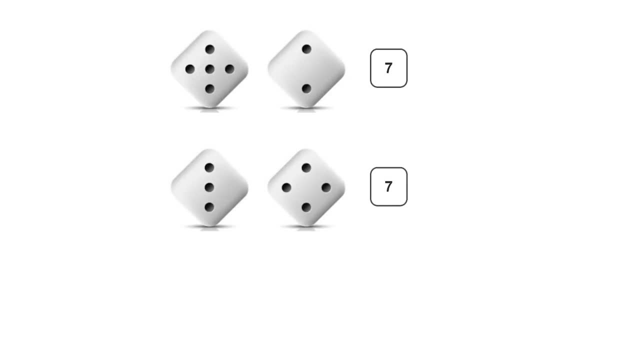 with two dice. you can either get a five and a two, a four and a three or a six and a one, But to roll a 12, you have to get a six and a six. There's only one way to do it, So there are more ways to get a. 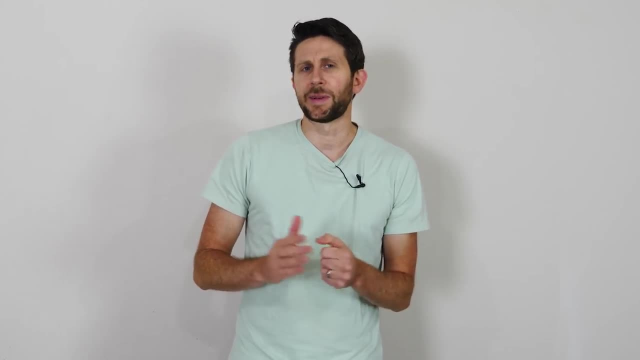 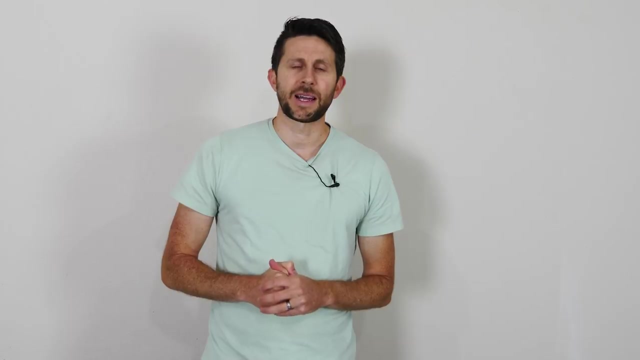 number that's right in the middle than those side numbers, So that's why the probability is much higher right in the middle. And thanks for watching another episode of the Action Lab. I hope you enjoyed it. If you did, don't forget to subscribe if you haven't yet, or hit the bell to be notified. 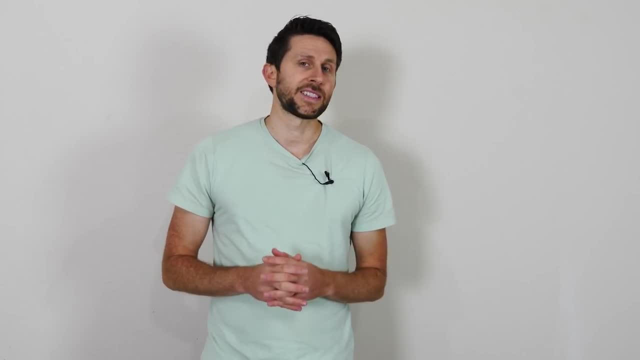 when I release my latest video And check out Action Lab Shorts, which is my second channel that I do videos similar to this one, but I do them in less than a minute And thanks for watching and I'll see you next time.